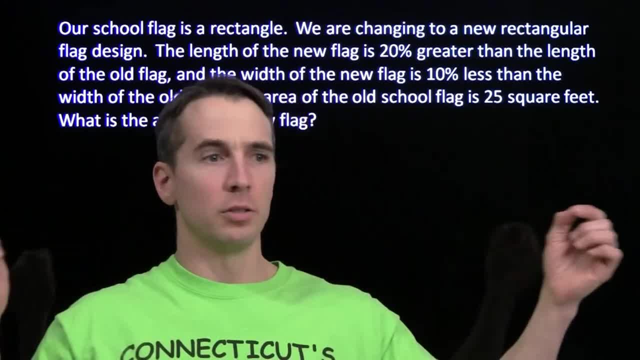 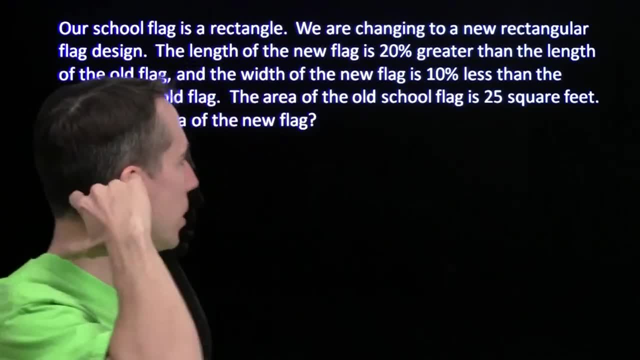 it's downstairs, I don't feel like going and getting it. I should have brought it up here, because then we could just measure the lengths and the width there and then we could figure out what the new flag's dimensions are going to be. But maybe we can figure this out without. 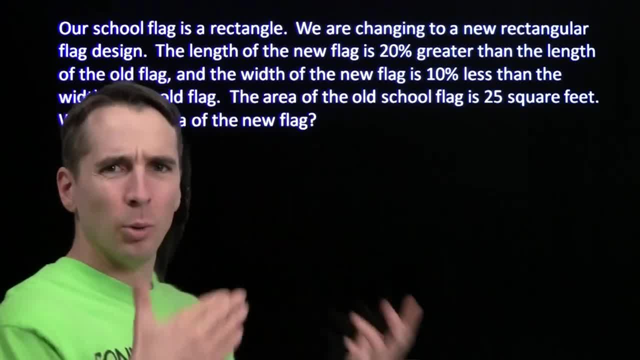 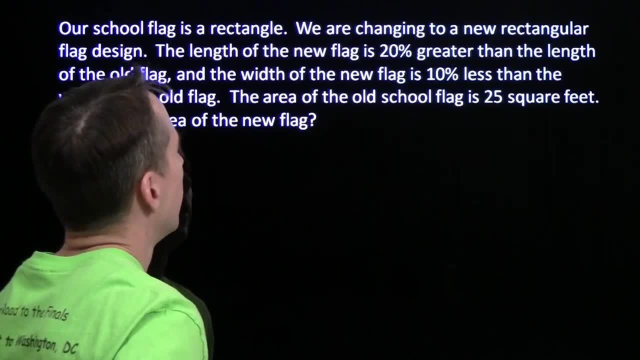 having the old flag, But it seems like I have to know what the dimensions of the old flag are to figure out what the dimensions of the new flag are. Oh, I'm confused. Well, you know, we're not going to solve the problem just by staring at it. so let's at least try something. Let's experiment. 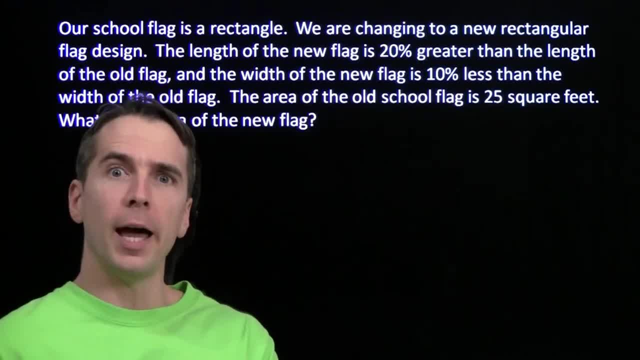 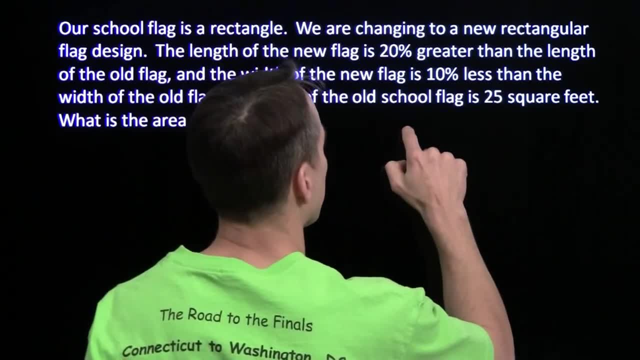 a little bit. Let's imagine we know what the dimensions of the old flag are. It's 25 square feet. We do at least know that. So let's- I mean that's a perfect square. Let's imagine the old flag's five by five, So we could start off with the old flag. 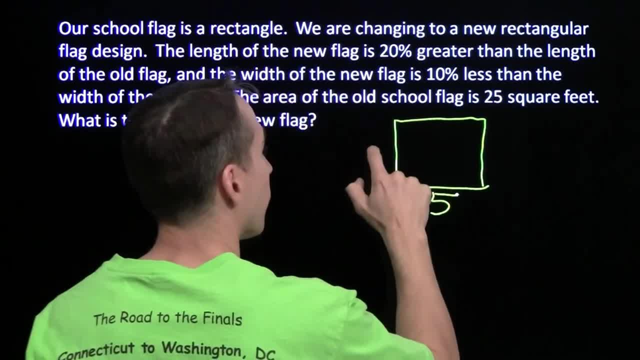 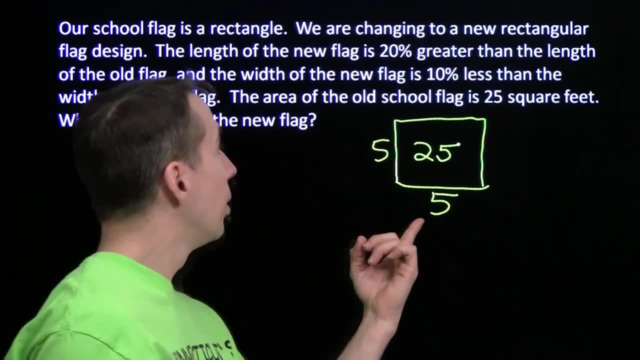 It's just a square, a five by five square, And of course the area then is 25, as planned. Now, if we increase the length of the flag by 20 percent, well, 20 percent of five, that's one-fifth of five, that's one. Increase it by one, that makes it six. Now we're going. 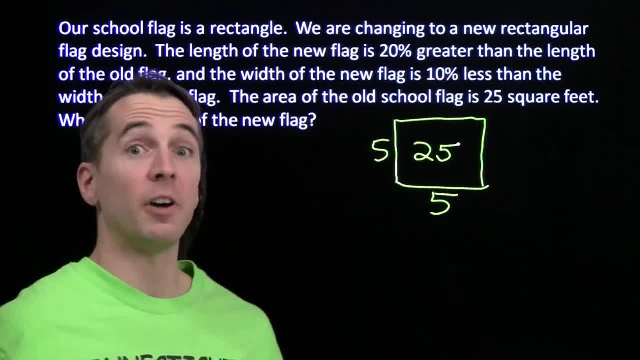 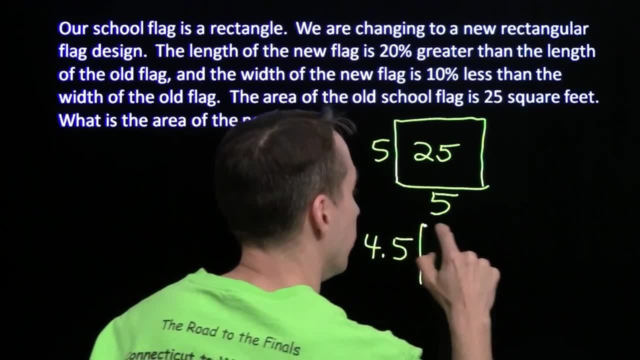 to decrease the width by 10 percent. 10 percent of five is 0.5.. Decrease by 0.5, you'll have 4.5 as the new width. So we have a new flag that's 4.5.. 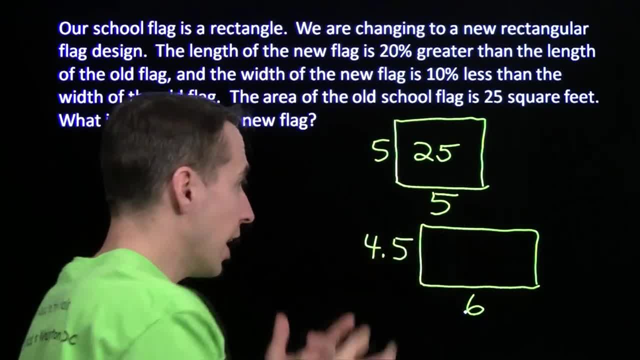 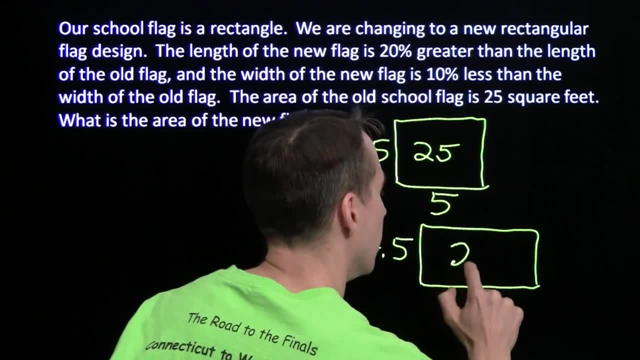 And 6 times 4.5, that'll give us the area of the new flag. 6 times 4 is 24.. 6 times 0.5 is another 3.. 24 plus 3 is 27.. Okay, that's good enough for a five by five flag, but what? 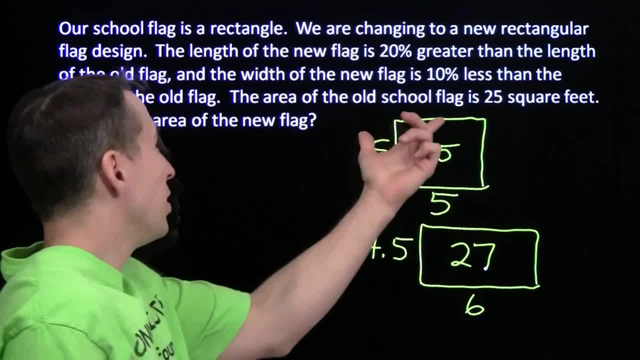 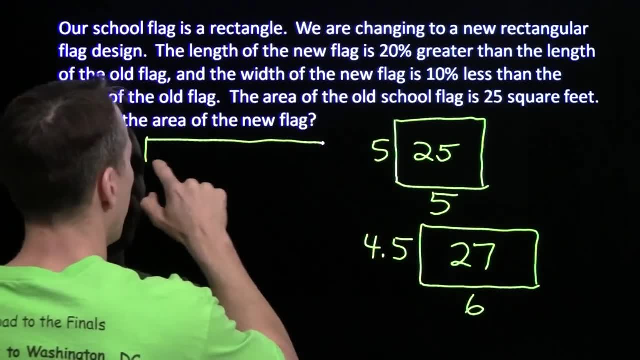 if the old flag's something different. I mean, 1 times 25 is 25.. So imagine we had a long skinny flag. Let's check that out. I don't think it's a 25 by one foot flag, but well. 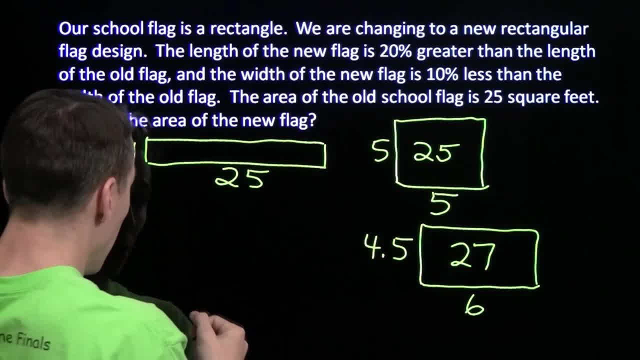 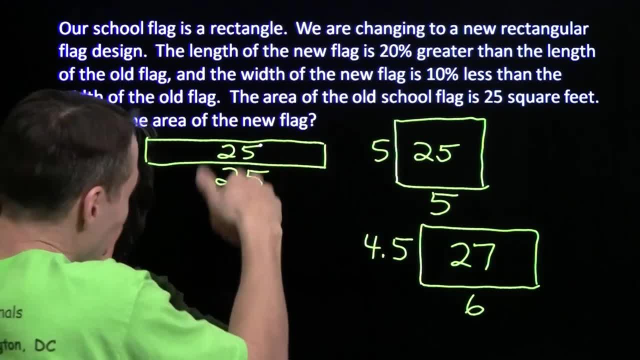 I'm experimenting here. Let's see what happens If we have a flag whose width is one length is 25 feet. that's a long, skinny flag. its area is 25.. Now let's check out what the new flag would look like. We increase the length by 20 percent. 20 percent of 25, that's one-fifth. 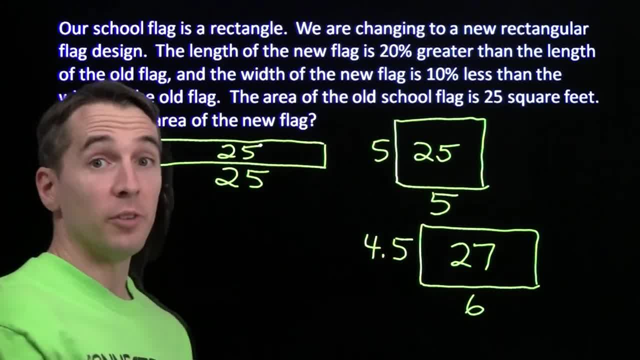 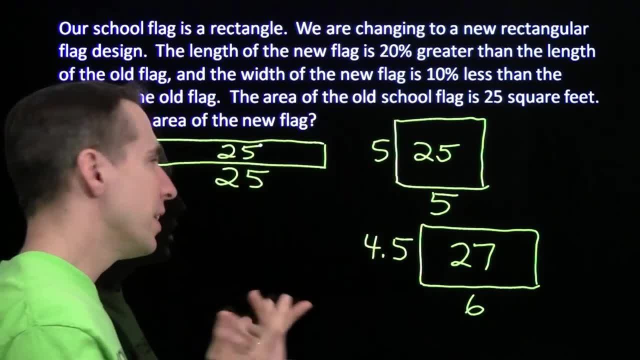 of 25 is five. so we're going to increase by five. from 25, that gives us 30.. We're going to decrease the width by 10 percent. 10 percent of one is 0.1.. Go down by 0.1, that gives. 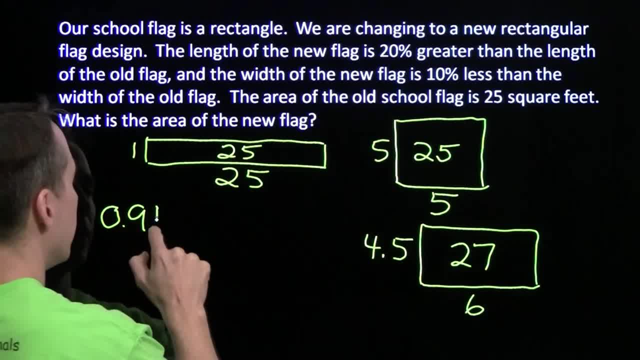 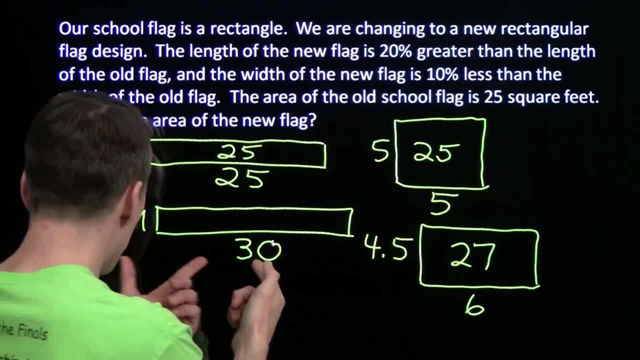 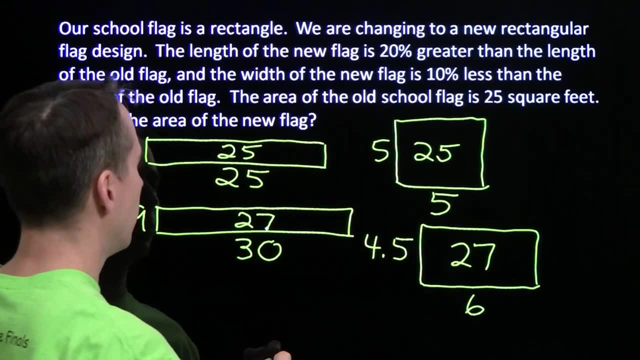 us 0.9.. So our new flag has a width of 0.9 and a length of 30. So its area is 30 times 0.9 is 27 again. Huh, I wonder if it always comes out to be 27,, no matter what the dimensions are, I mean. 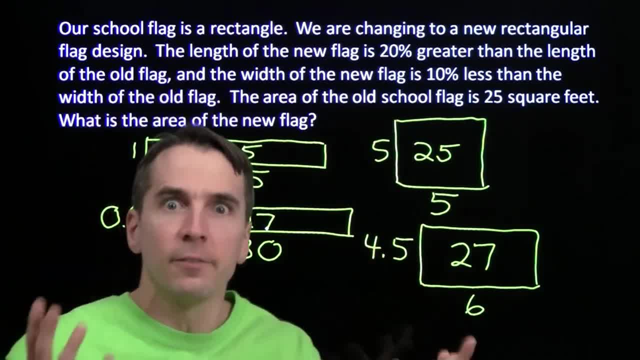 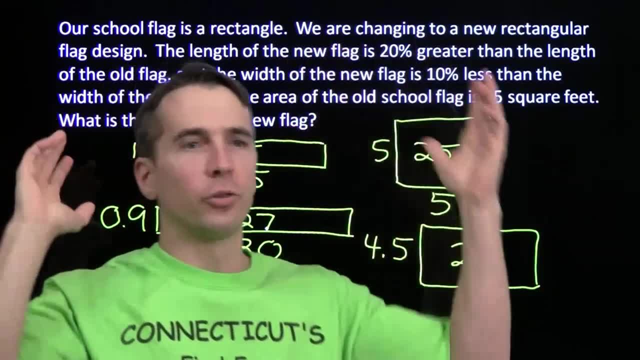 well, we can't check every possible case right. That'll literally take forever, because there are infinitely many possibilities. It could be, you know, length of 10, width of 2.5, or all sorts of things. You know it could be infinitely many possibilities. How? 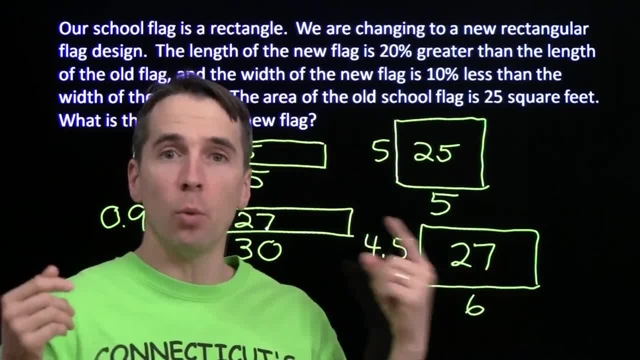 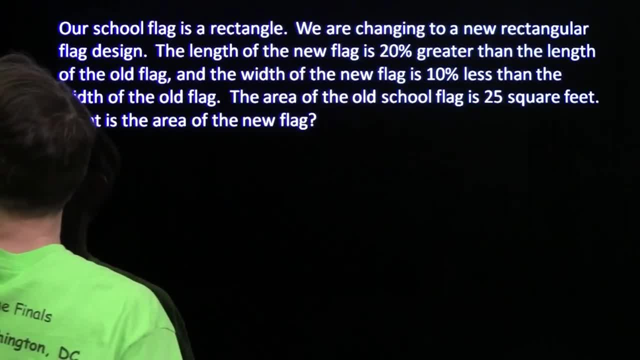 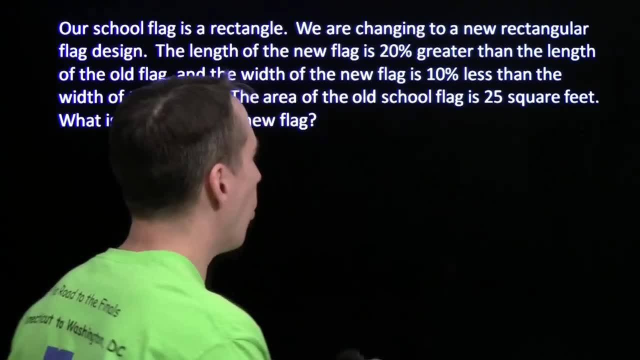 can we possibly check infinitely many possibilities at one time? Variables- Variables are great for that. Let's try that. Instead of picking numbers for our length and our width, let's just use variables. That'll let us check all the possibilities at one time. We'll start. 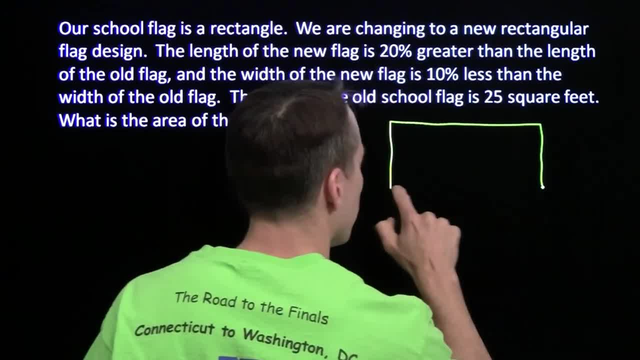 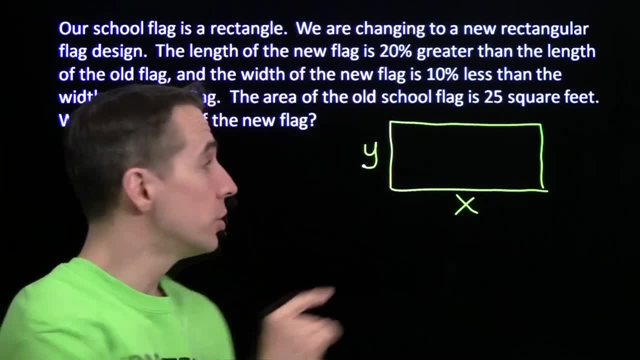 off. Here's my school School flag. The length is x, The width is y. We don't know what x and y are, but we do know the area of the flag is 25 square feet. So we know that x times y is 25.. I'm 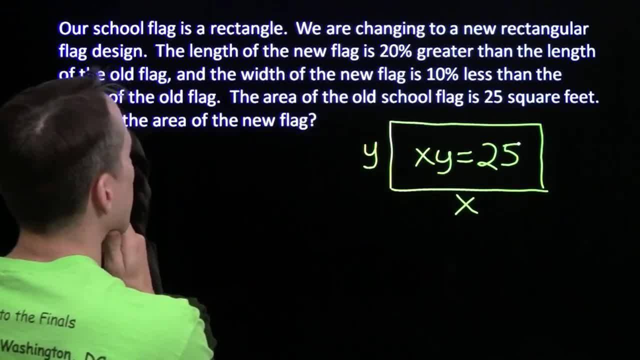 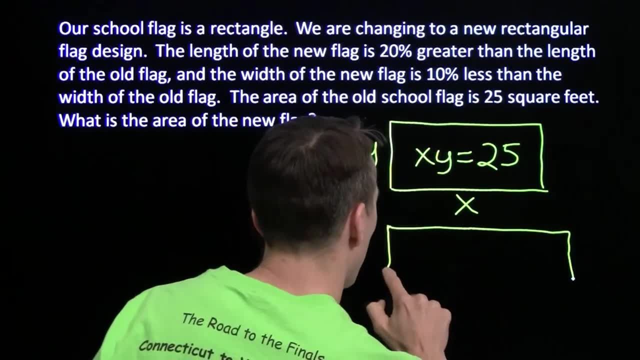 going to go ahead and write that down. Now let's see What's next. Oh, that's right, New flag, New flag. We want a little bit skinnier. We're reducing the width, We're increasing the length. 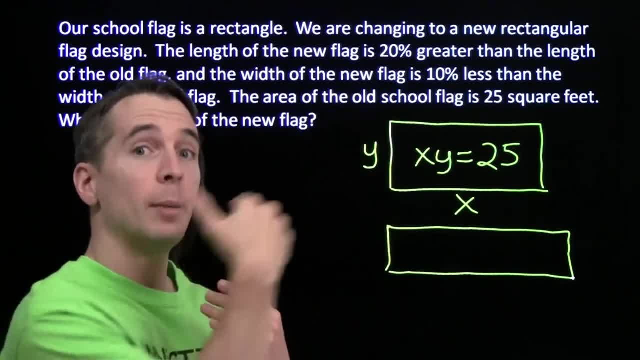 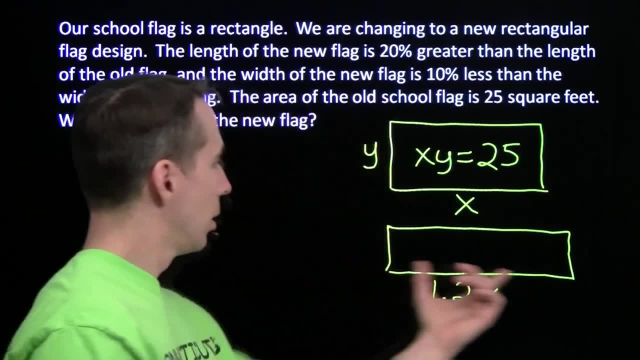 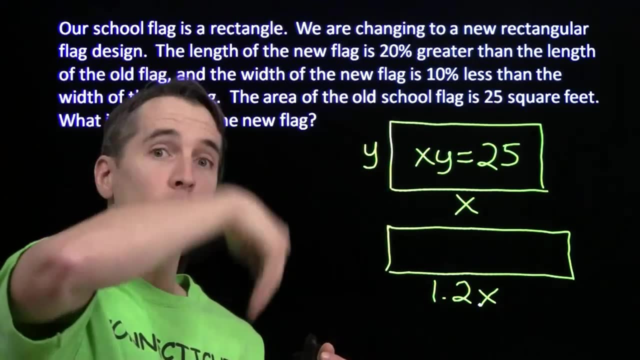 The original length is just x. We increase by 20%, We add 0.2x on and we get 1.2x for the length of the new flag And the width. Well, we go down by 10% from the original. The original was y. 10% of y is 0.1y. We go down 0.1y. We. 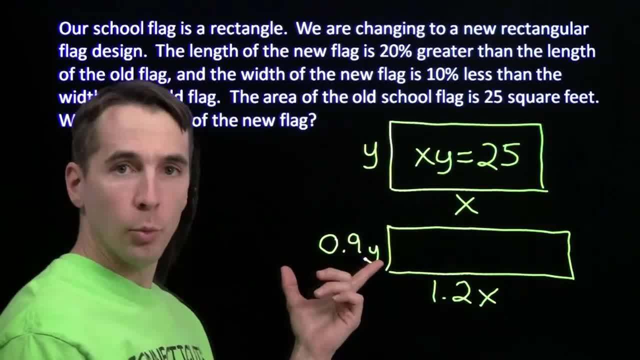 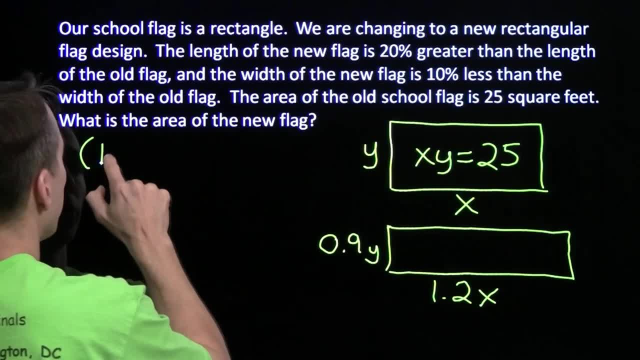 have 0.9y for the width, And then we need the area of this new flag. We take the product of the length and the width, We multiply 1.2x, 1.2x, 1.2x. 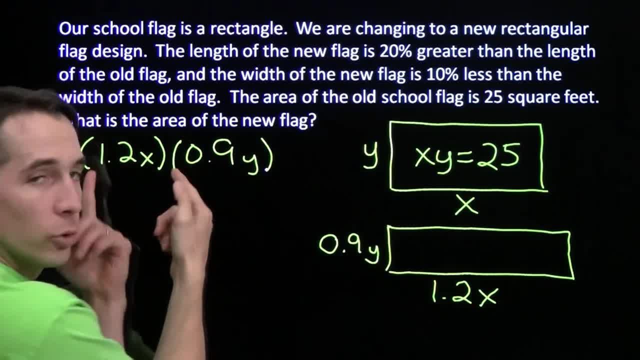 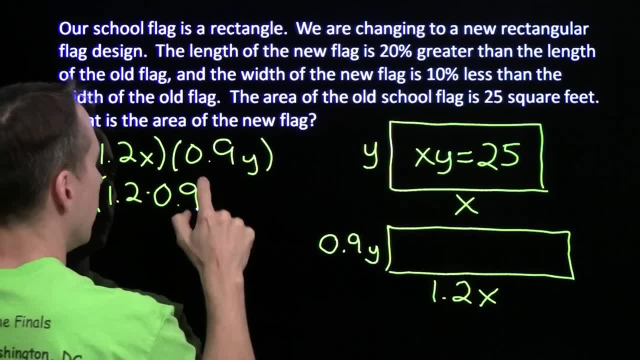 1.2x And 0.9y. I'll go ahead and group the 1.2 and the 0.9.. 1.2 times 0.9.. And we'll put the x and y together. 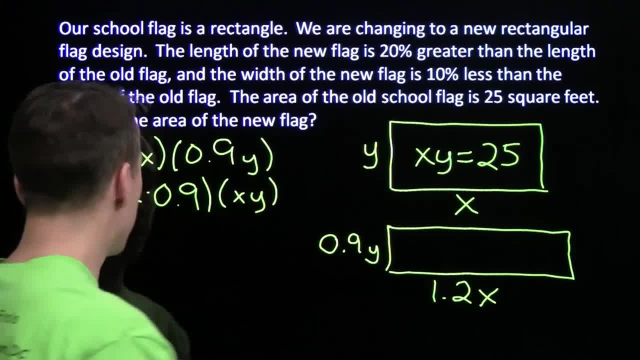 And 1.2 times 0.9.. 12 times 9 is 108.. So 1.2 times 0.9 is 1.08.. And oh, x times y. I don't know what x is. 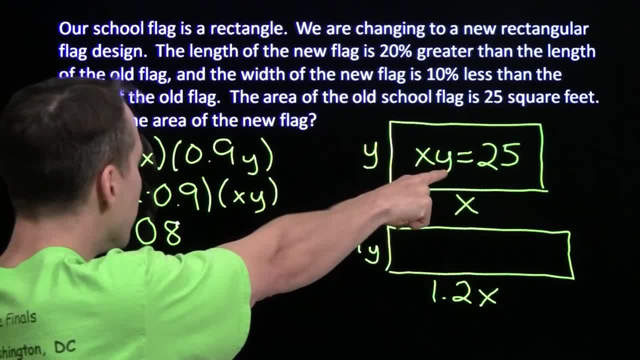 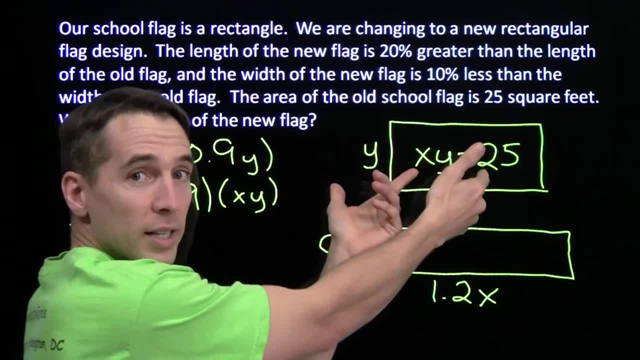 know what y is, but wait, We do know what x times y is. Check out. this is why we write down things that we know. Once we figure something out, we know that x times y is 25.. If we hadn't? 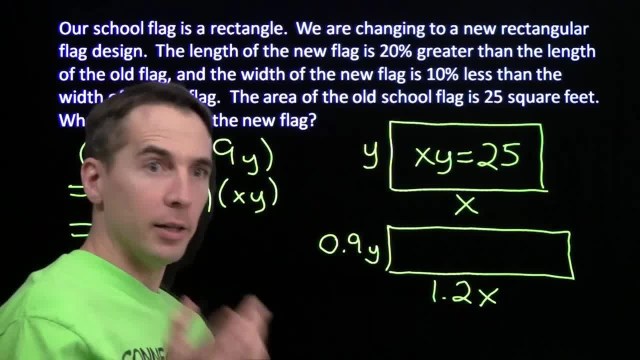 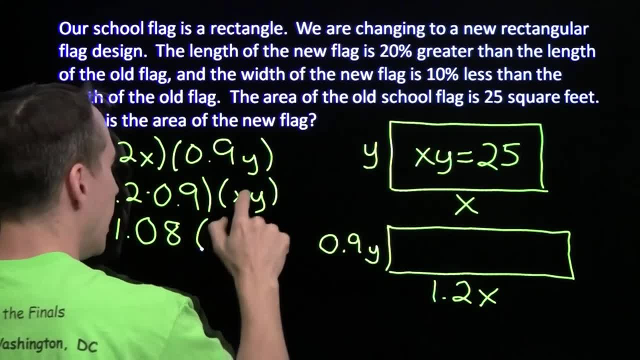 written that down there. we might have forgotten it- At least I would have forgotten it, Maybe you wouldn't have, but it's sitting right there. So we're looking for x times y. We have it written right over there so we can bring x times y equals 25 right over here. 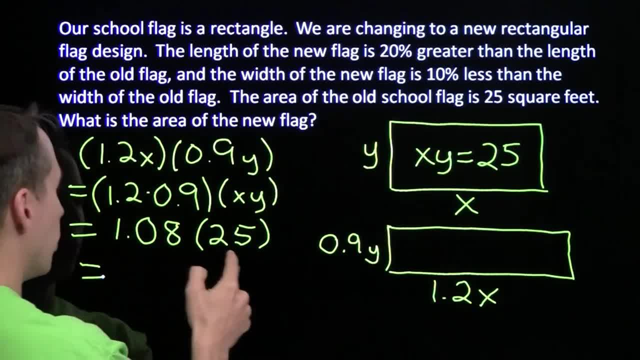 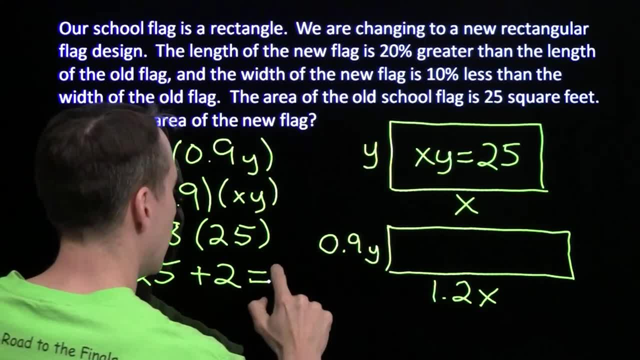 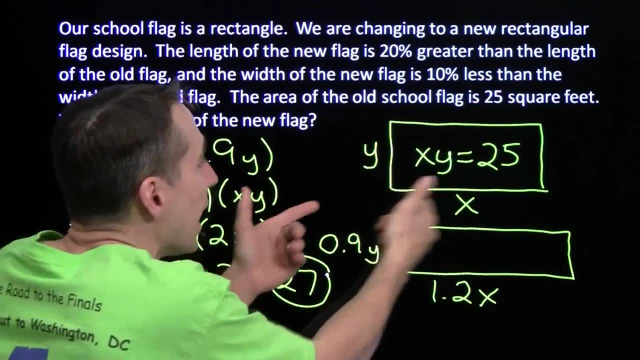 Our answer is 25 times 1.08.. 25 times 1 is 25.. 25 times .08, that's another 2.. So the area of the new flag is 27 square feet, and it doesn't even matter what the dimensions. 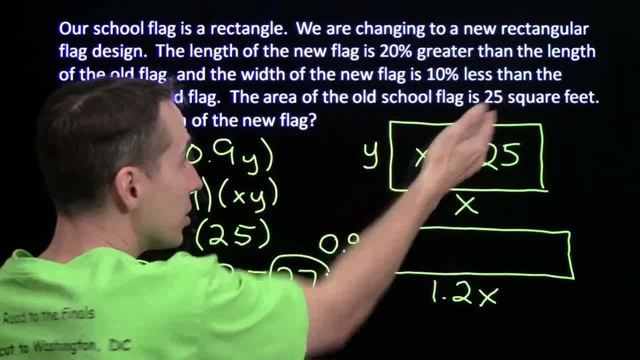 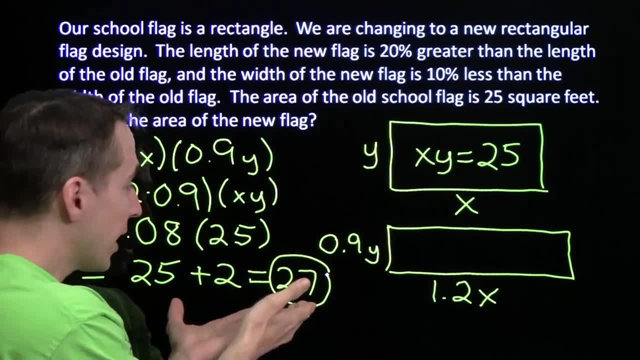 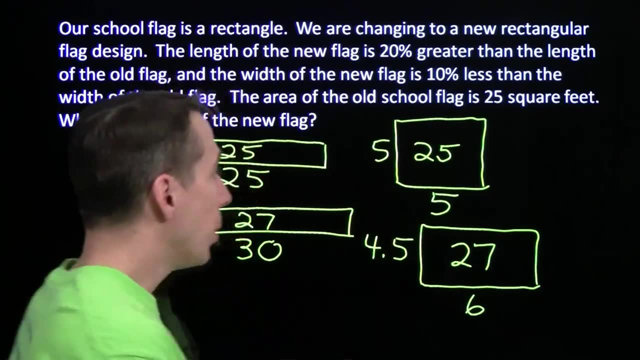 of the original flag are As long as the area is 25 square feet to begin with. we increase the length by 20%, we decrease the width by 10%. the area of the new flag is going to be 25.. Now let's recap real quick Our key steps. In the beginning, we didn't know what to do. 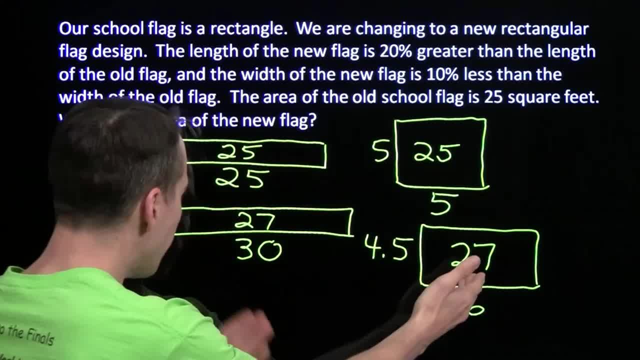 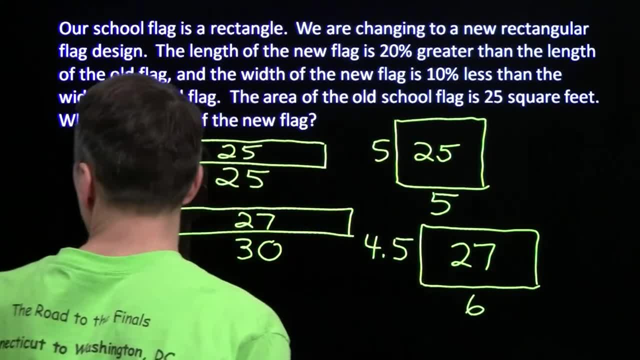 but we didn't just stare, We experimented and we discovered something interesting. It looks like the area would always be the same, but we had to check every possibility at once. Variables are good at that. So if you have an unknown, if you have something you don't- 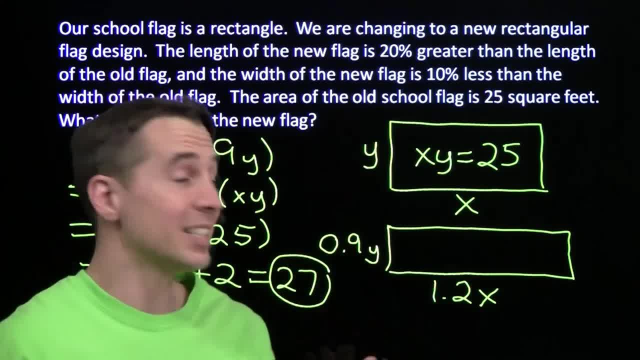 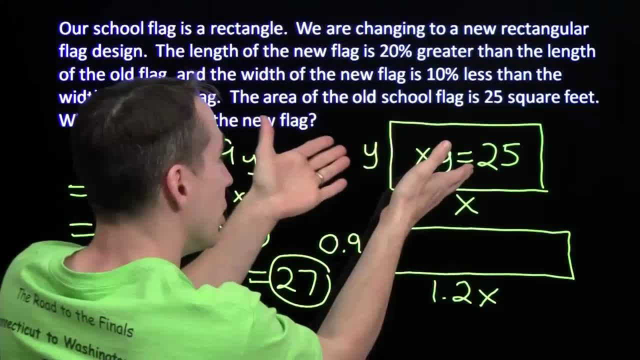 know in a problem, assign a variable And then, when you find things that you do know, write it down, just in case it'll become useful later. And once you write down everything, you take all these words, you turn it into math and 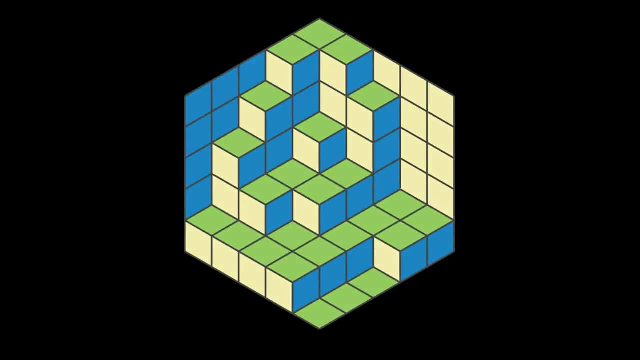 you work through that math and then finally you're done.